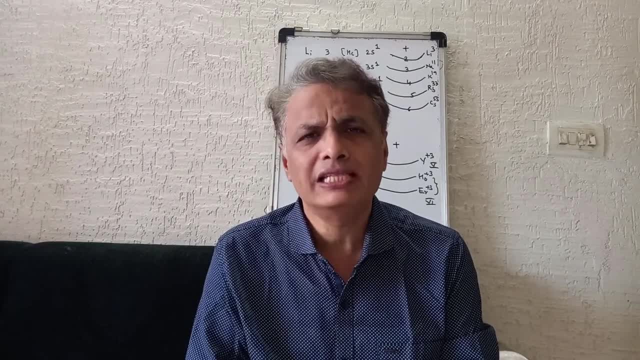 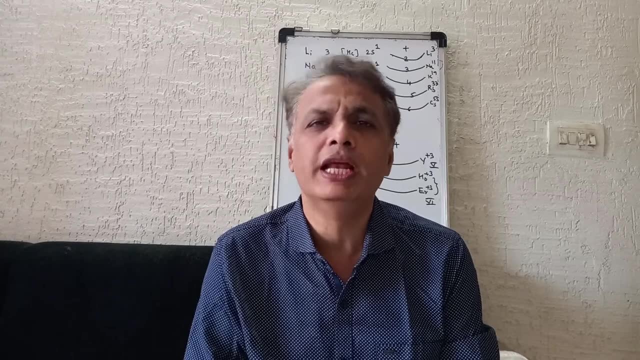 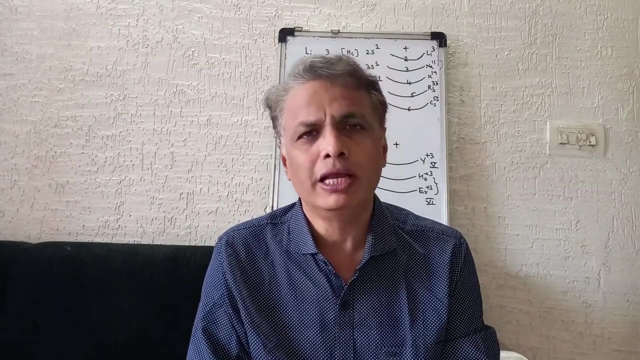 normally in the group. as atomic number increases, atomic radia increases because new entering electron takes position in new orbital. Normally in a group, when we talk about group number 1 to 18, normally in the group. as atomic number increases, atomic radia increases because new 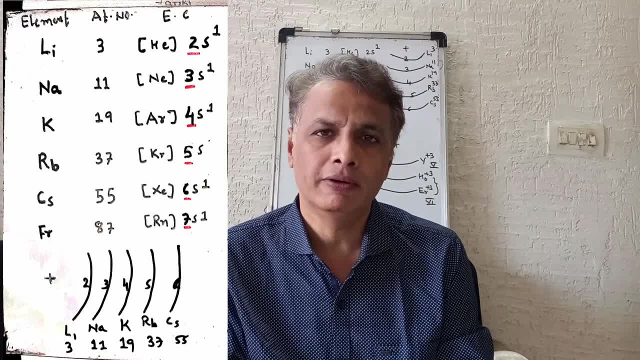 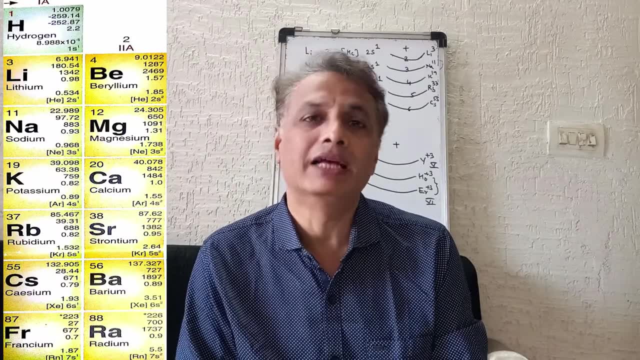 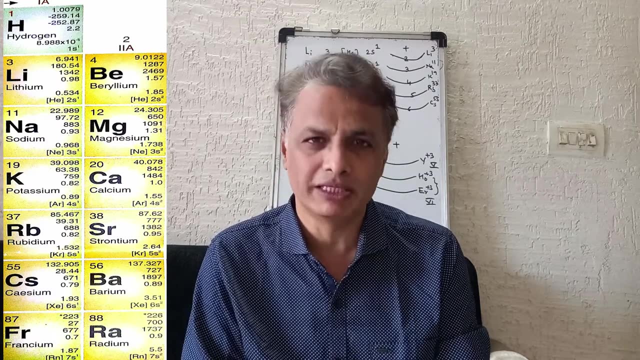 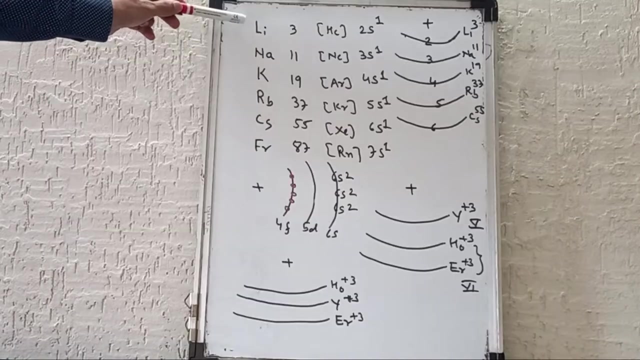 entering electron takes position in a new orbital. Let us understand this thing with the example of Alkali metal. Alkali metal, you can remember with the help of Helen Cabrassier-Farrar. These are alkali metal: Lithium, Sodium, Potassium, Rubidium, Cesium and Francium. 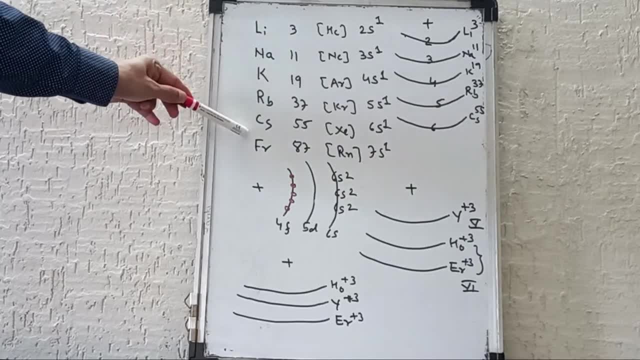 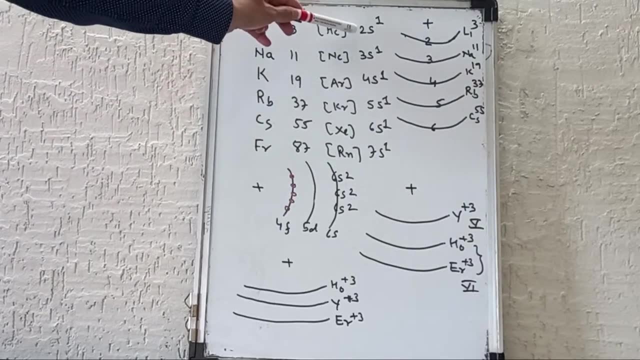 You can remember with the help of this trick, Helen Cabrassier-Farrar, These are the atomic number 3,, 11,, 19,, 37,, 55,, 87, and these are the principal quantum number: 2,, 3,, 4,, 5,, 6, 7.. 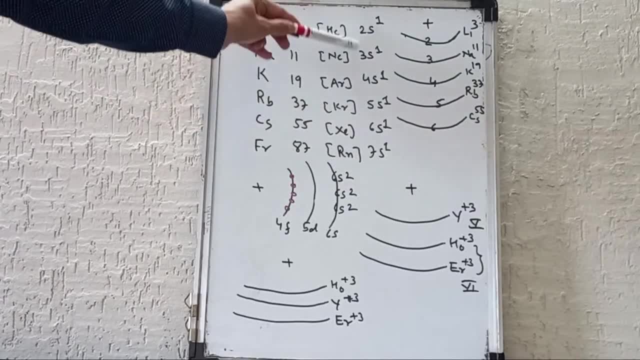 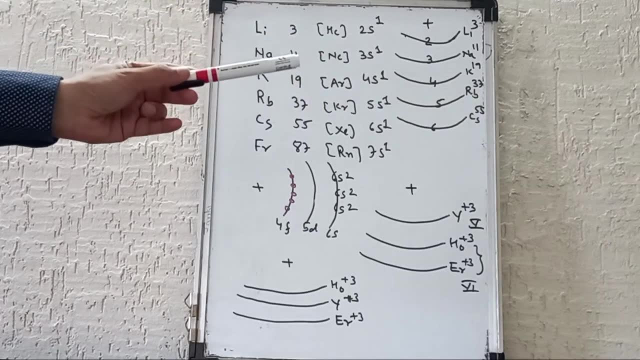 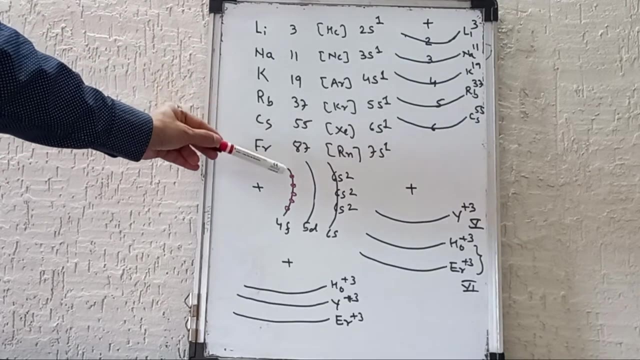 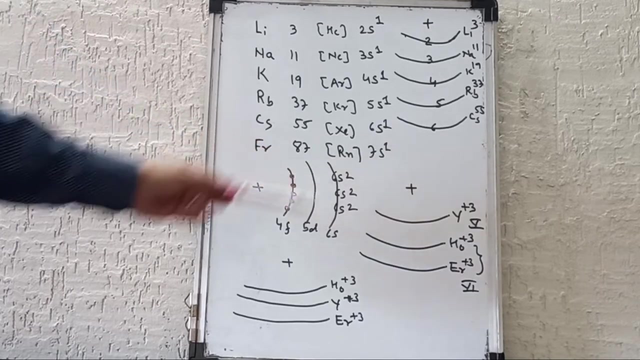 So as atomic number increases, principal quantum number also increases and therefore distance of electron from the nucleus increases and therefore atomic radia goes on increasing. But in case of lengthened element, new entering electron takes position in 4M energy level. So number of electron in outer energy level remains the same. 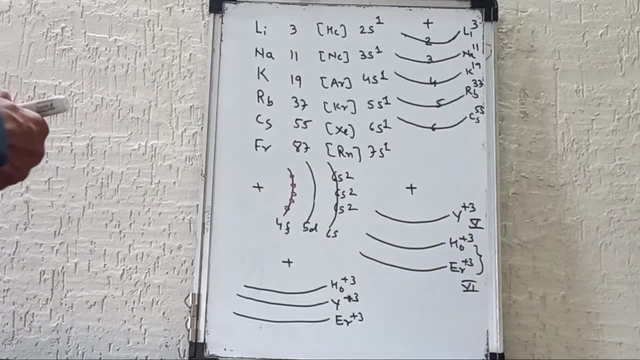 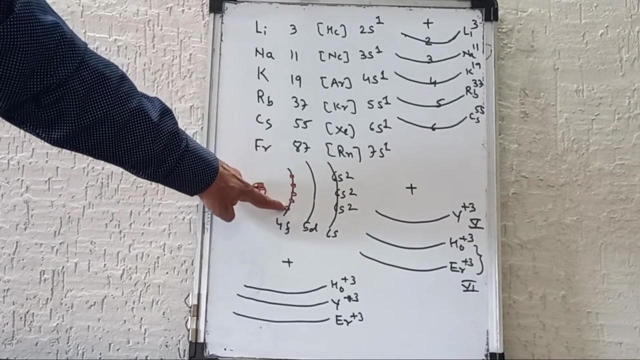 Moreover, as atomic number increases, this nuclear charges also increases, This nuclear charges also increases and therefore atomic radia goes on decreasing. This type of decrease in atomic radia it is known as lengthened contraction. I am repeating: In the case of lengthened element, new entering electron takes position in 4M energy level. 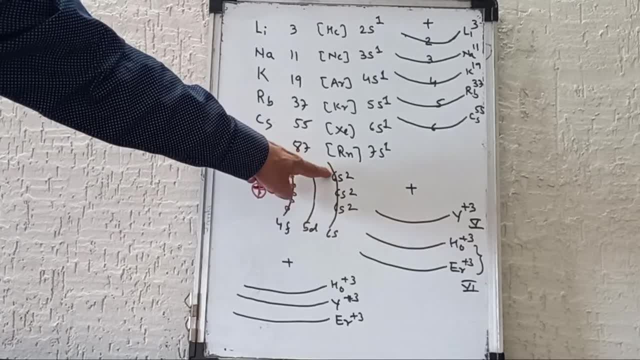 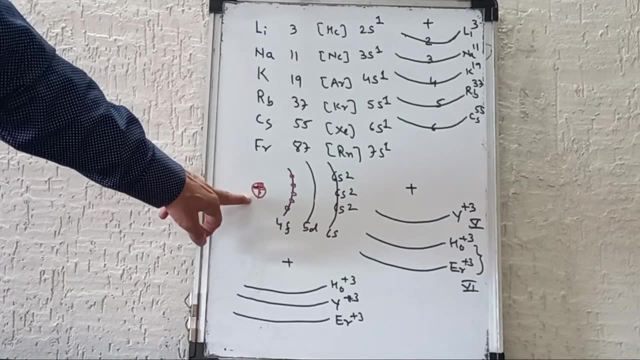 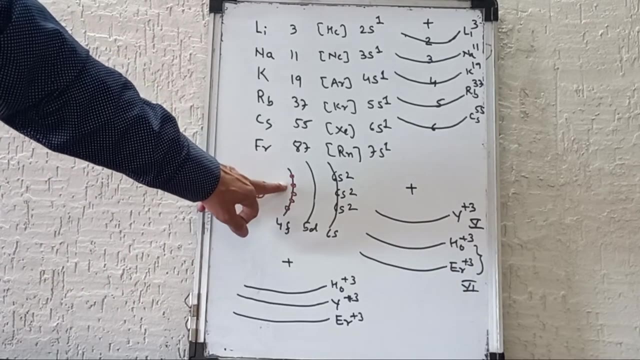 instead of outer energy level. So number of electron in outer energy level remains the same. Moreover, as atomic number increases, nuclear charges also increases. Here new entering electron takes position in 4F energy level. This 4F energy level is having diffuse shape, and therefore electron of F orbital does not 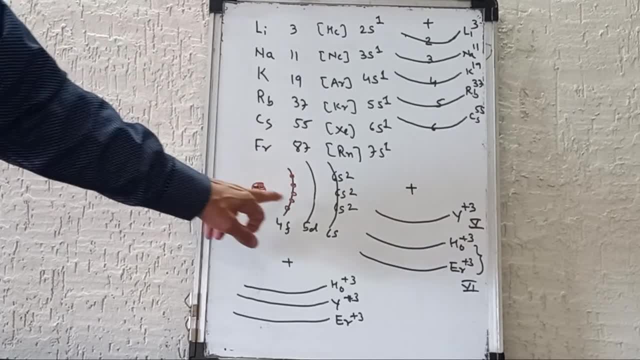 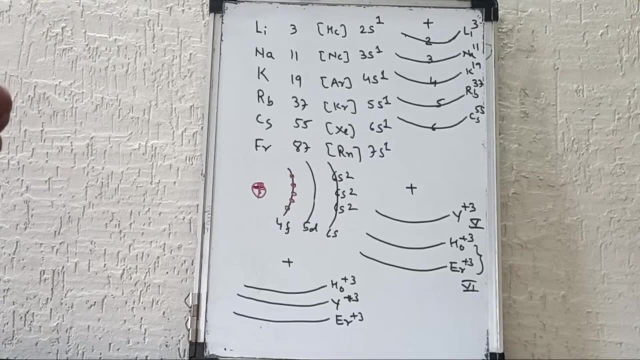 see 6S electron, and therefore, as nuclear charges increases, it also decreases. It attracts electrons and therefore atomic radia goes on decreasing. This type of decrease in atomic radia it is known as lengthened contraction. Now let us discuss the effect of lengthened contraction. 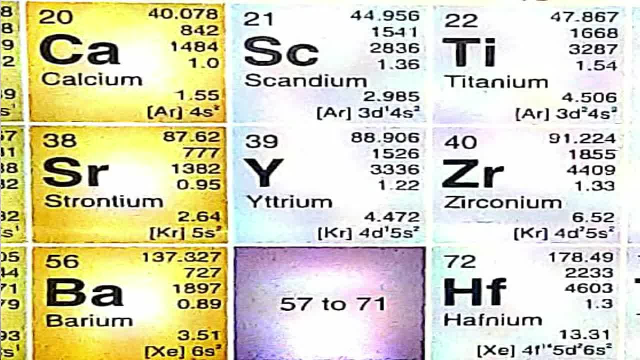 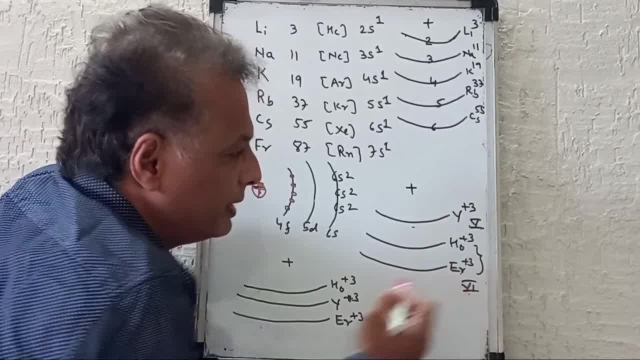 Yttrium is a fifth period element and Holmium and Erbium are sixth period element Due to lengthened contraction. H is the fifth element, So H is the sixth element. So H is the sixth element, So H is the fifth element. 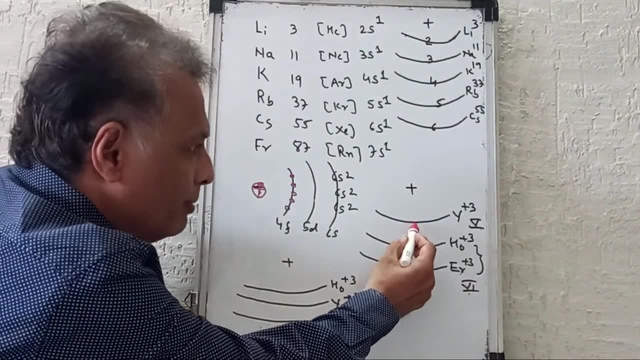 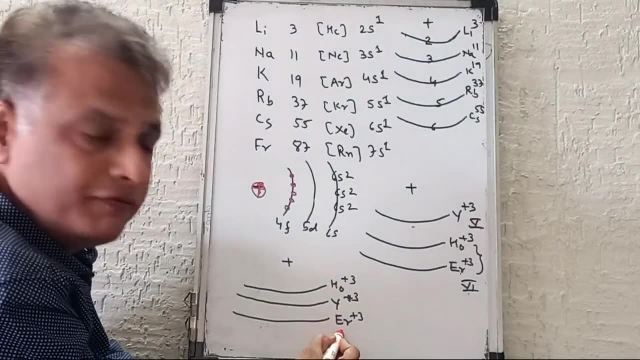 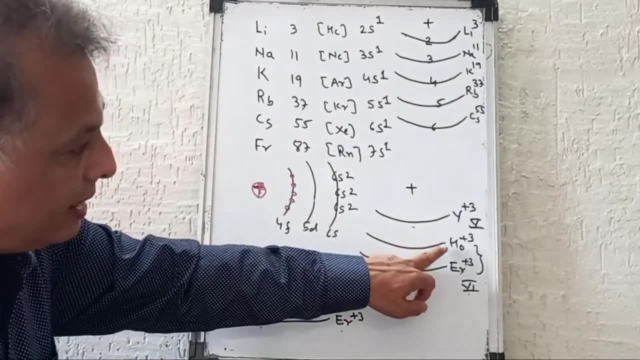 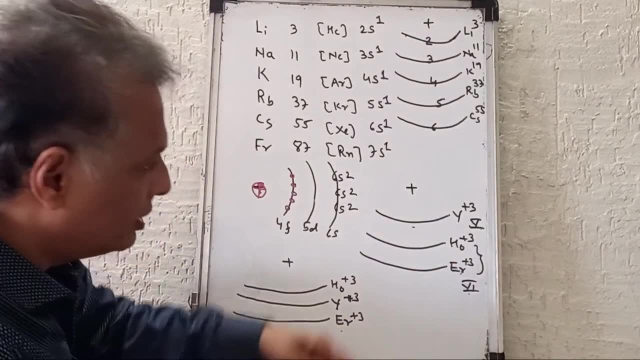 Yttrium is a fifth period element and Holmium and Erbium comes under sixth period, that is, lengthened element. Now, due to lengthened contraction, atomic radius of Yttrium remain unchanged, but atomic radius of Holmium and Erbium goes on decreasing. 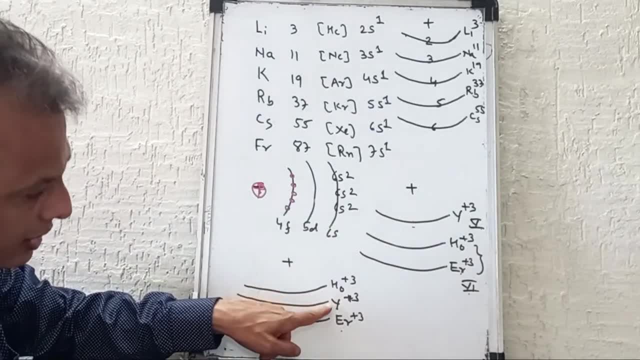 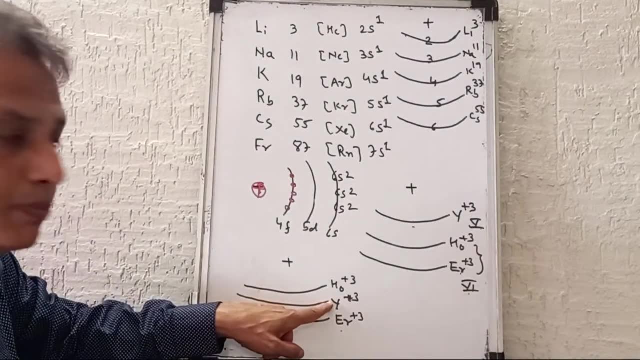 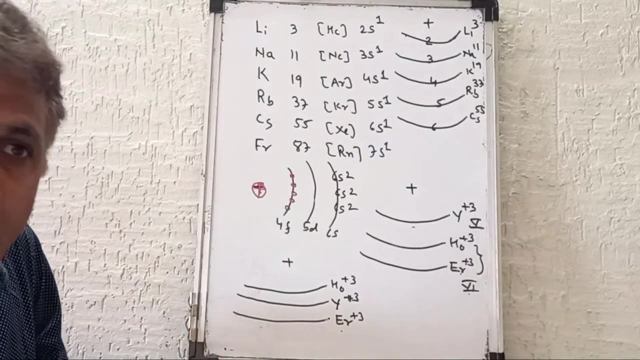 And therefore atomic radius of Yttrium comes between atomic radius of Holmium and Erbium. So, in spite of being the member of fifth period, Yttrium is found with lengthened element. Now, due to lengthened contraction, atomic radius goes on decreasing. Due to lengthened contraction, atomic radius goes on decreasing And the difference between two consecutive lengthened element is lengthened. So the difference between two consecutive lengthened element is less than 0.01 Angstrom. Difference between two consecutive lengthened element is 0.01 Angstrom. Moreover, as atomic number increases, atomic radius goes on decreasing. Therefore, atomic radius of lengthened element are quite near to the fifth period element And there would be possibility of fifth period element between two consecutive lengthened element And therefore it is very difficult to separate lengthened and lengthened. 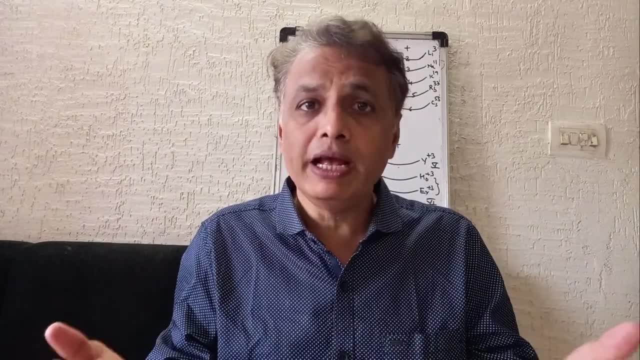 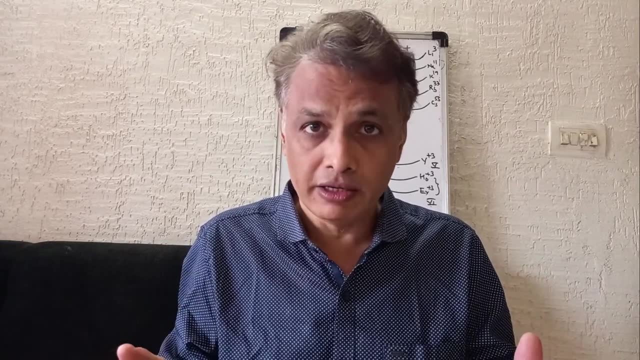 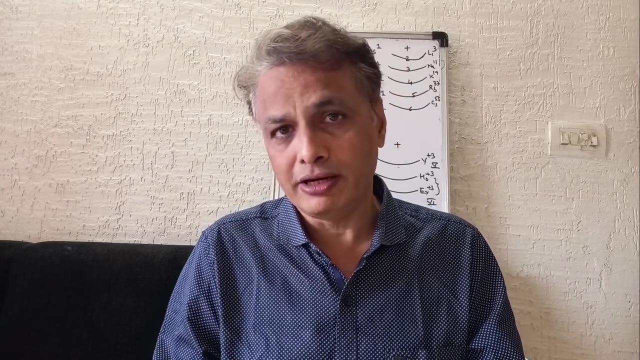 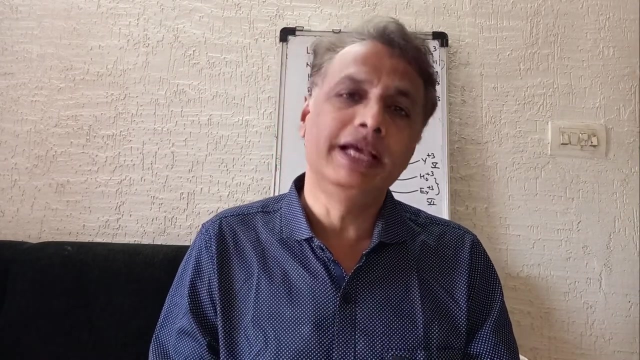 It is very difficult to separate lengthened element from fifth period element as well as lengthened element from one another, And therefore separation of lengthened is very difficult And it can be separated by either spectroscopic method or ion exchange method. Third thing: as atomic number increases, atomic radius goes on decreasing. 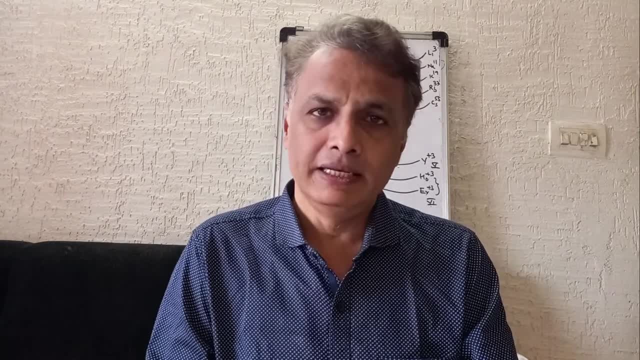 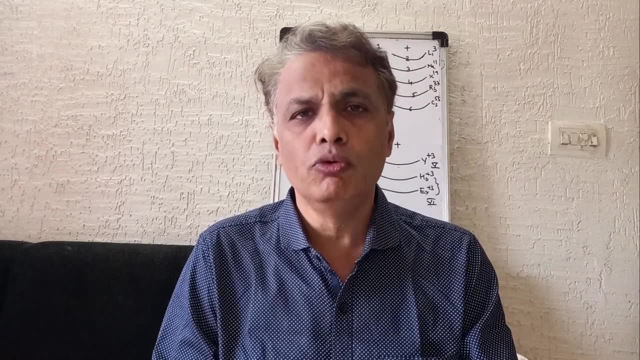 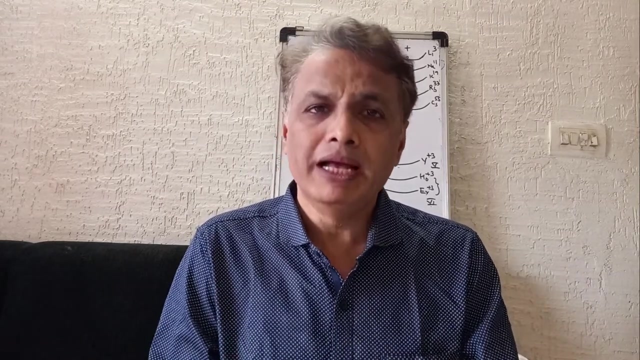 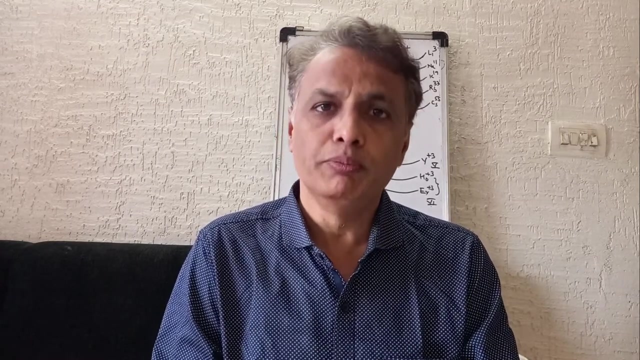 Point number four: basicity Is with which electron is removed. it is called basicity Is with which electron is removed. it is called basicity If ion is bigger in size. Therefore that electron is removed very easily. Therefore it acts as strong base. As we move from Lentenum to Lutetium, atomic radius goes on decreasing As Lentenum is largest in size and Lutetium being smallest in size, And therefore Lentenum forms strong base. Hydroxide of Lentenum forms strong base. While Lutetium hydroxide forms weak base, As we move from Lentenum to Lutetium, atomic radius goes on decreasing. Therefore, Lentenum is largest in size and Lutetium is smallest in size, But as we refer electronic configuration or atomic radius of Lutetium, 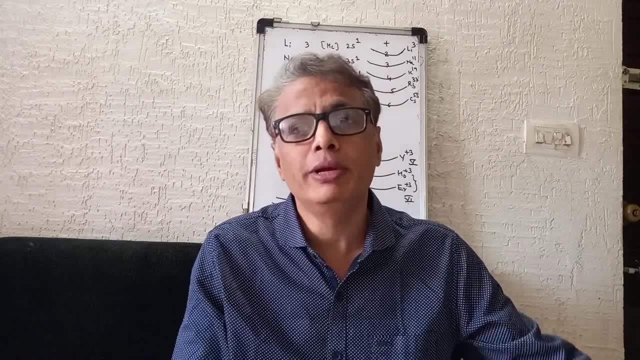 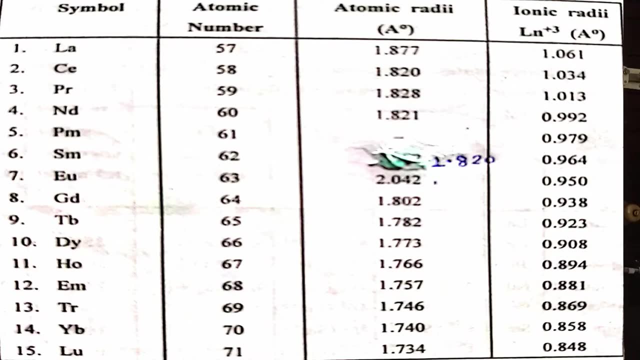 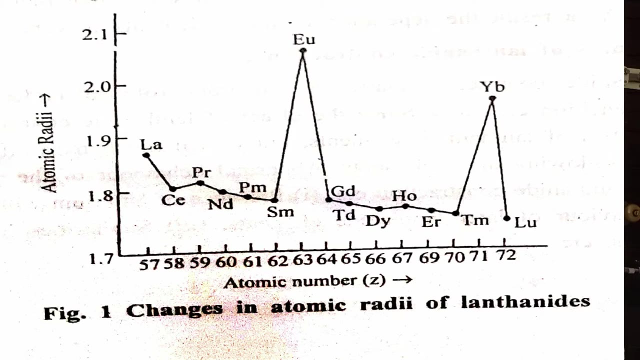 Atomic radius of Europium does not decrease than that of Samarium. Atomic radius of Europium does not decrease than that of Samarium. Reason is that electronic configuration of Europium is 4F7- 5D06S2.. It has half-filled electronic configuration. 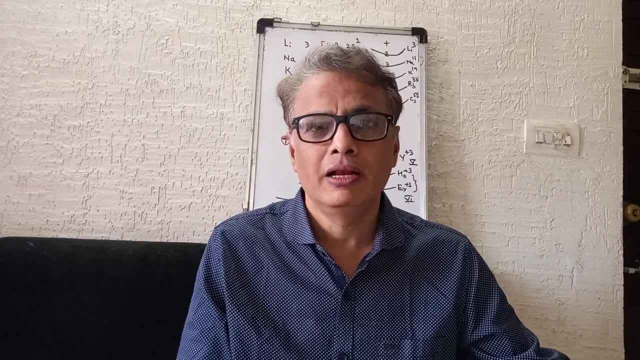 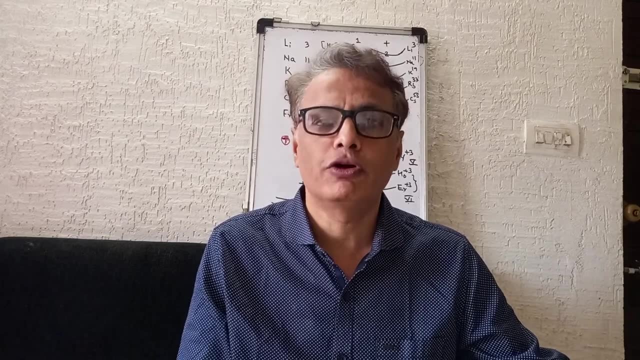 So electron try to repel And therefore electron try to remain as far as possible from one another And therefore nucleotide is not visible. And therefore nucleotide is not visible And in general the molecular charges do not attract electron of 4F energy level. And therefore size of Europium does not decrease than that of Samarium. Now we are going to discuss basic property of lanthenide element. As we move from Lentenum to Lutetium, atomic radius goes on decreasing And therefore, as Lentenum is largest in size and Lutetium being smallest in size, 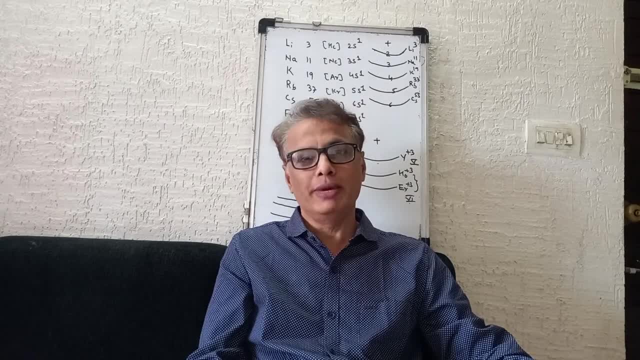 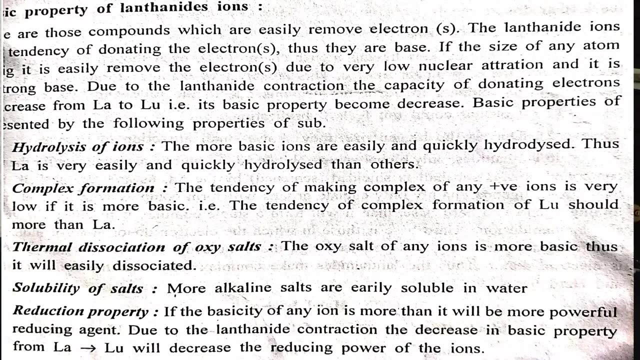 hydroxide of lanthanum is strong base, while hydroxide of lutetium is weak base. The more basic ions are easily and quickly hydrolyzed. Thus, lanthanum is very easily and quickly hydrolyzed than other ions. The 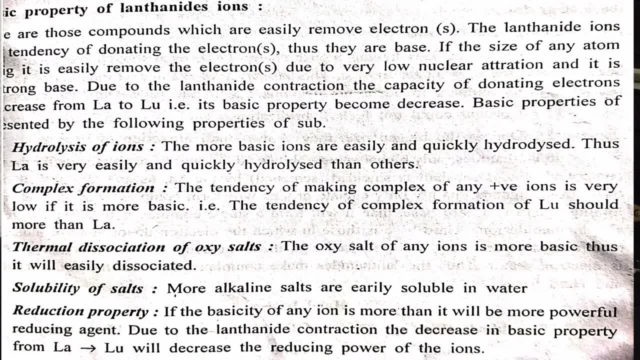 tendency of making complex of any positive ion is very low if it is more basic and therefore the tendency of complex formation of lutetium should be more than lanthanum. If basicity of any ion is more than it will be more powerful reducing agent Due to lanthanite contraction, reducing power of 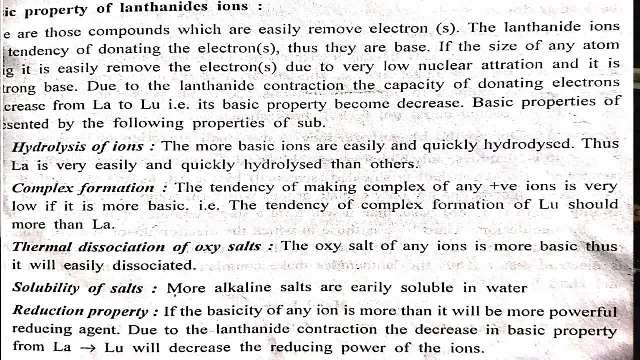 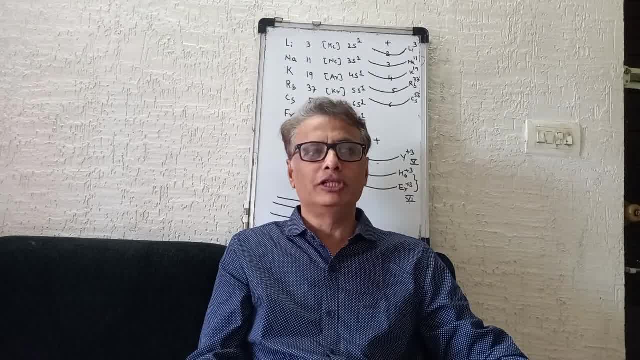 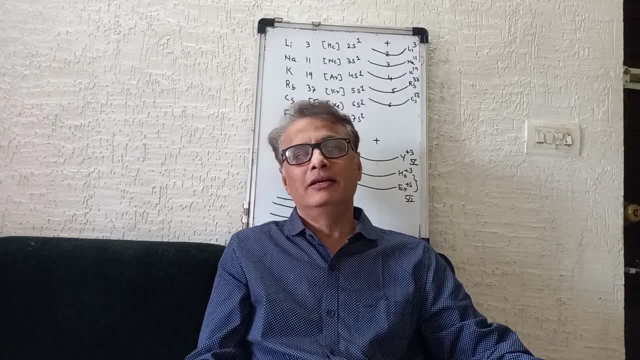 reducing power decreases from lanthanum to lutetium. Now we'll discuss regarding capacity of complex formation of lanthanite. The capacity of complex, complex formation of lanthanite should be minimal for the use of lutetium, and formation of lanthanide is very less. F-orbital could not feel hybridization. due to bigger in size, they show small attraction to the ligand.